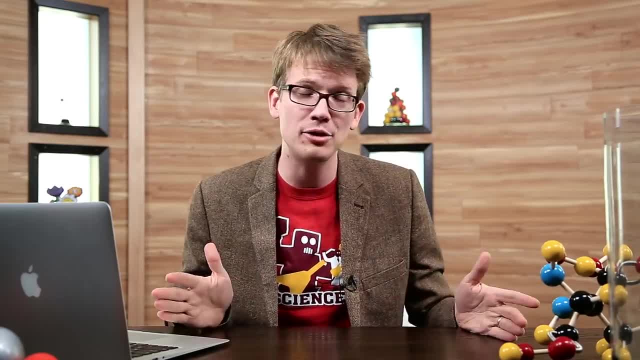 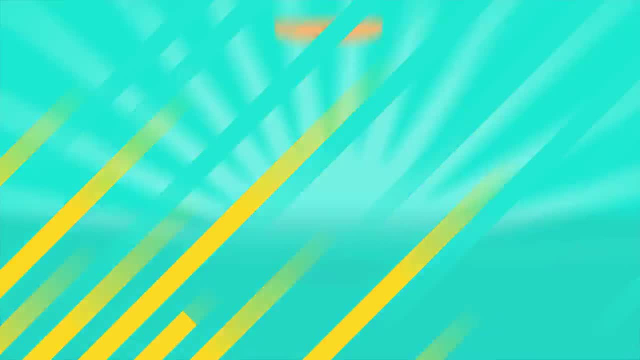 opposition to the disorder and are, in fact, often impossible to achieve. The very act of putting one system in order requires that other systems become disordered. Think of it this way: Your lunch was composed of an extremely ordered set of molecules. 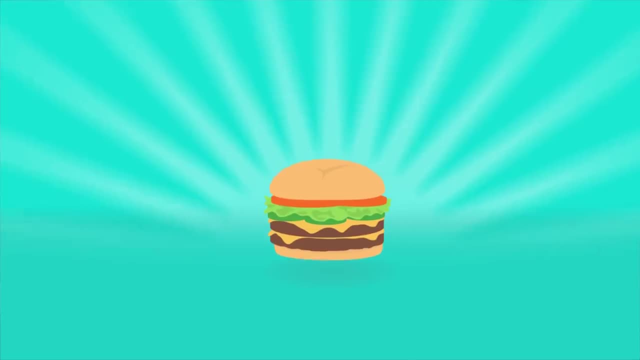 and it gave you the energy to clean up your house, maybe. And it had to be broken down into less-ordered nutrient molecules for you to do that- Carbohydrates, proteins and lipids- and those molecules were broken down even further as they were converging. 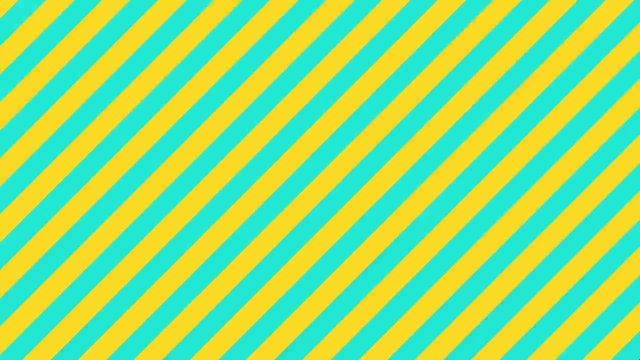 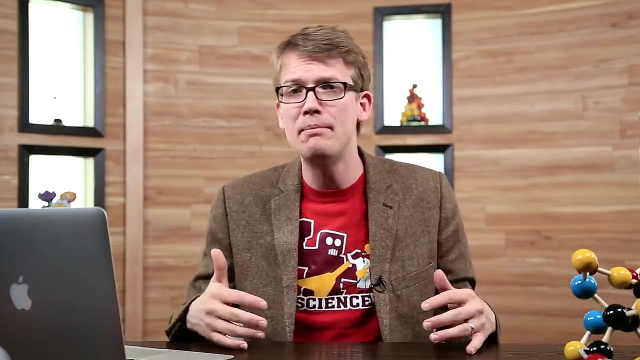 They were converted to energy in your cells and then your body used some of that energy to power your muscles as you cleaned your house. But much of that energy was used to do things like keep your heart beating and breathe and make sweat, and some of that was lost to the surroundings in the form of random movement. 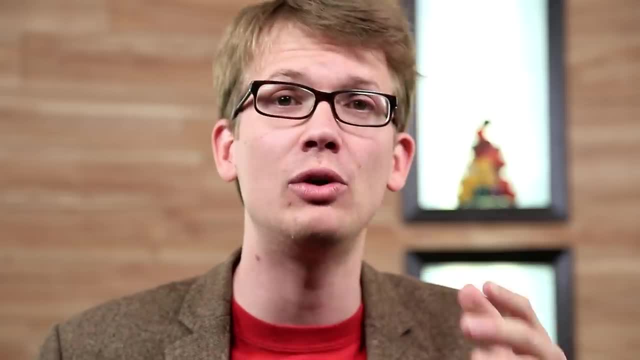 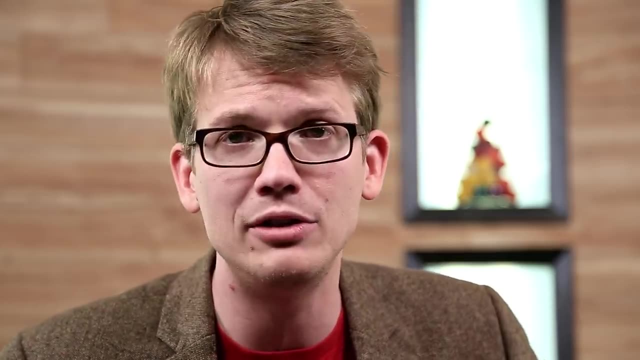 and, most importantly, heat. By the time you're finished, your house may be orderly, but the remains of your lunch molecules are all over the place, and that's only one of the many systems that became less orderly while you worked. So, yes, cleaning your house in fact increased the overall disorder of the universe. 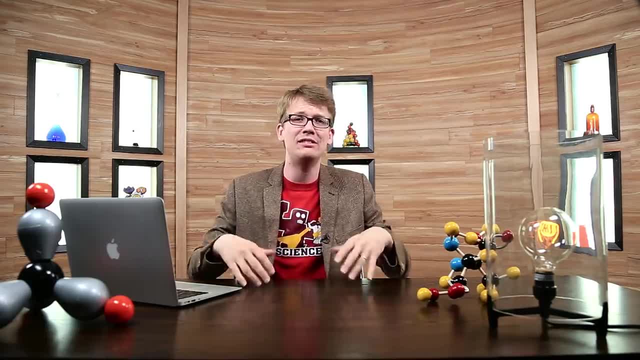 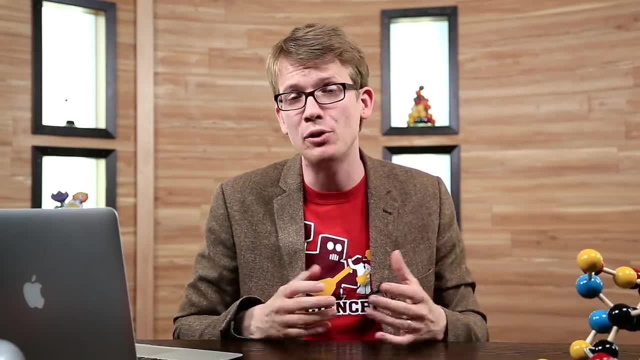 Next time someone gives you a hard time about the state of your house, you can tell them that, Obviously, disorder is a pretty big deal in the universe and that makes it a pretty big deal in chemistry. So scientists have a special name for it: entropy. 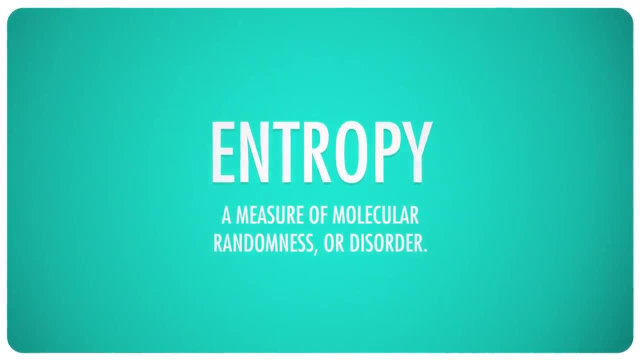 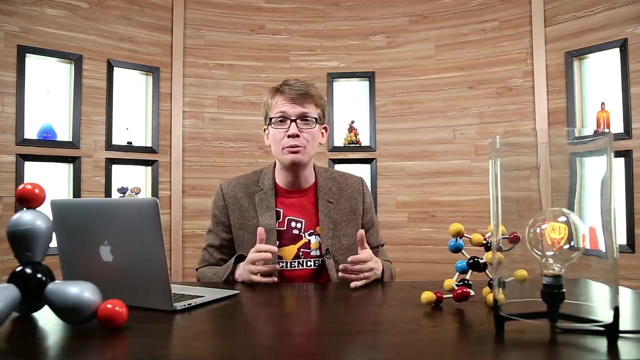 Entropy is a measure of molecular randomness or disorder, and even though people complain about the disorder in their lives, it's not all bad news. Entropy helps make chemical reactions possible and it helps us predict how much useful work can be extracted from a reaction. We all have to live with disorder, so you might as well. 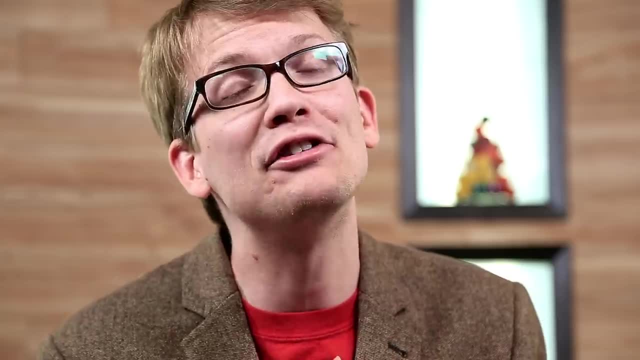 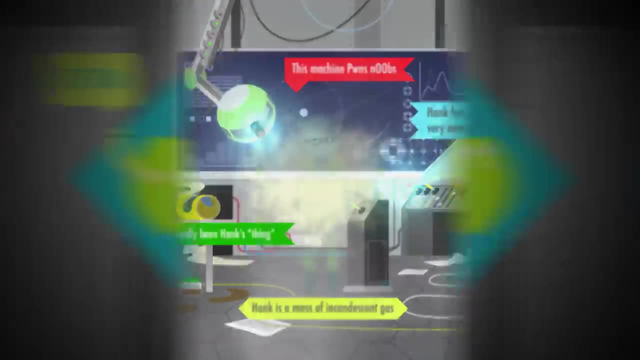 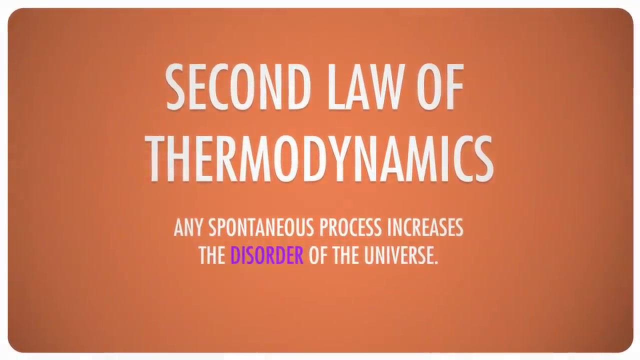 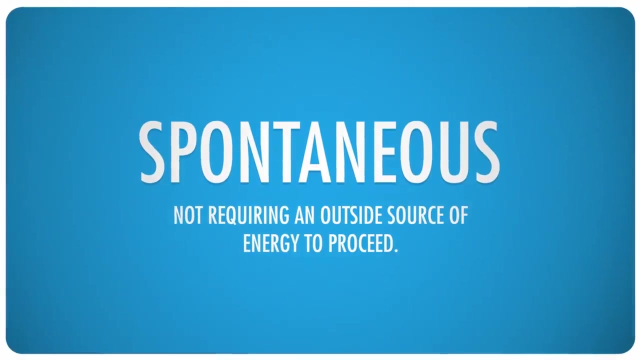 stand it for the next ten minutes. I want you to embrace the chaos. So what does the second law of thermodynamics mean when it says any spontaneous process increases the disorder of the universe? Spontaneous simply means a process that doesn't need outside energy to keep it going. 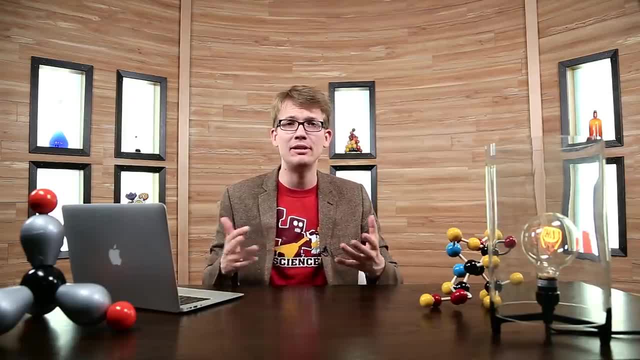 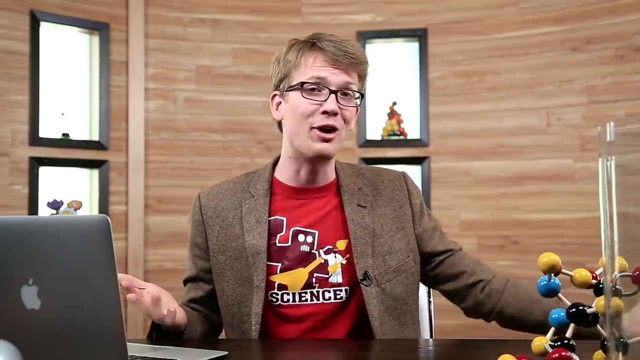 And it goes the other way too. Anything that increases the disorder of the universe happens spontaneously. That doesn't mean disorderly things will always happen, though Other factors may interfere. The reaction to change a diamond into graphite, for example, would be thermodynamically spontaneous. It wouldn't have to be forced along by outside energy, But the bonds in the diamond are so stable that, essentially, it never gets started. Lots of other chemical reactions are like this too. So even though we sometimes think of spontaneous as meaning, sudden and impulsive like the. 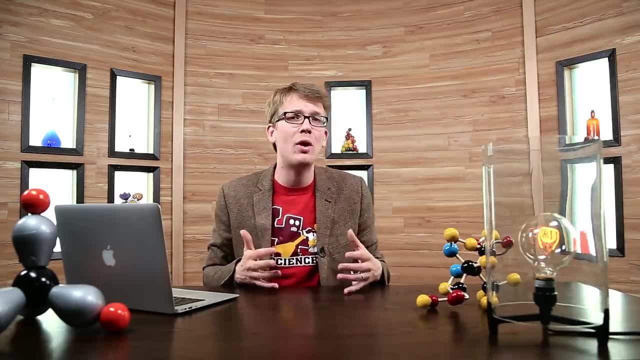 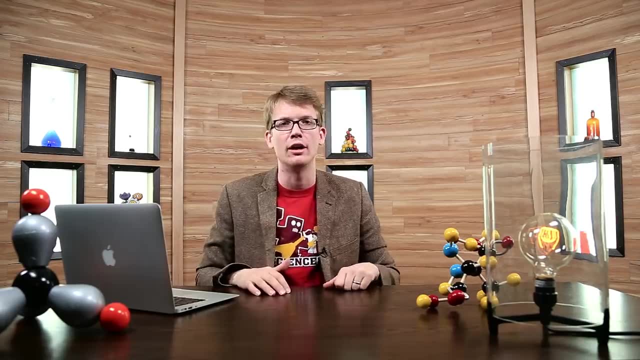 majority of Maul lip-piercings in chemistry, spontaneous, doesn't tell you how quickly something happens. It only means a reaction is thermodynamically capable of happening without outside energy to move it along. Though, come to think of it, I imagine that spontaneous lip-piercings cause a fair amount. 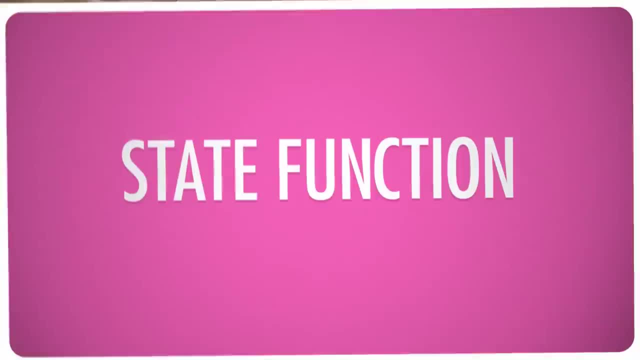 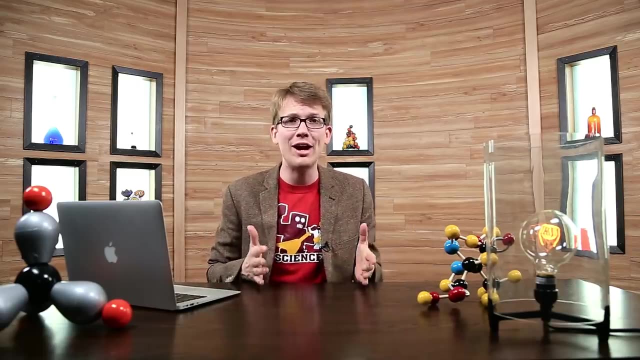 of disorder as well, especially upon arriving home. Entropy is another state function. It doesn't depend on the pathway the system took to reach its current state. So even though we can't measure the entropy of reactants or products directly, we can. 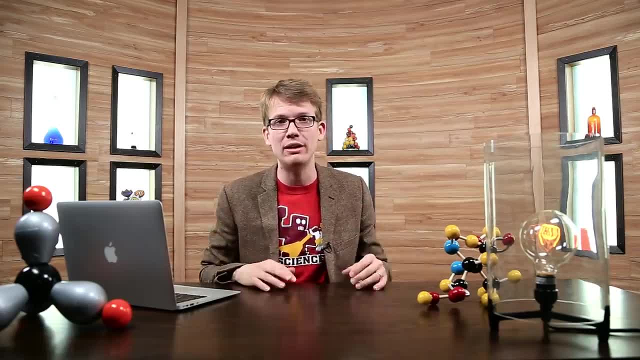 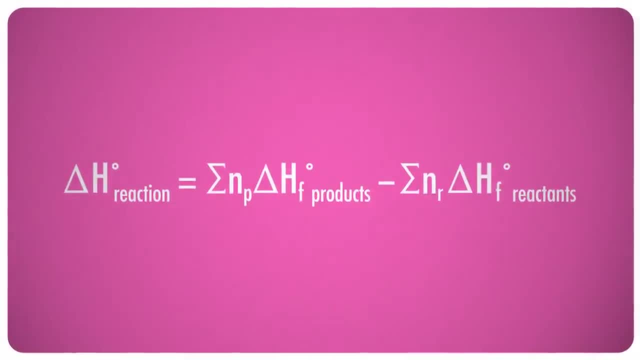 calculate them. We can also calculate the change in entropy that occurs during a reaction, exactly like we can for the change in enthalpy, by subtracting the sum of the reactant values from the sum of the product values. In other words, the formulas look exactly the same, just substituting S, which, for some, 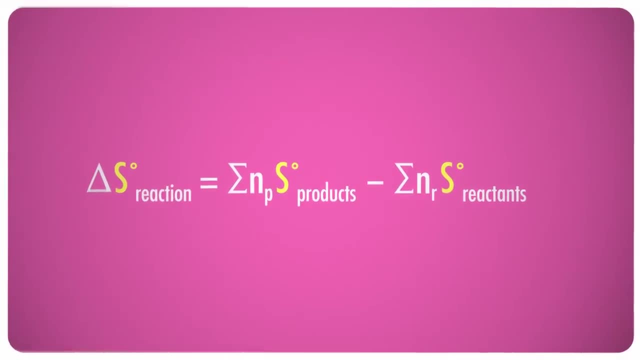 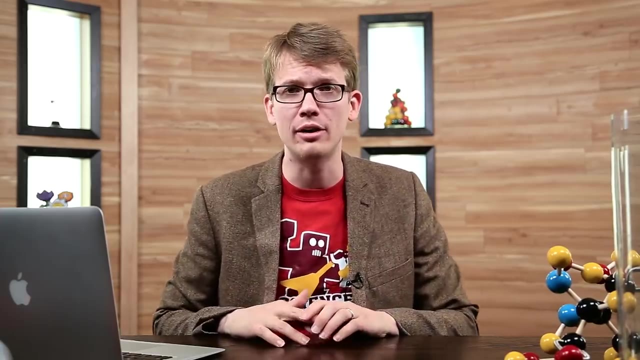 reason is used to denote entropy for delta HF. Notice that we drop the deltas on the right side of the formula because we know absolute values for entropy of individual reactants and products. We keep the delta on the left because we're calculating the change in entropy that occurs. 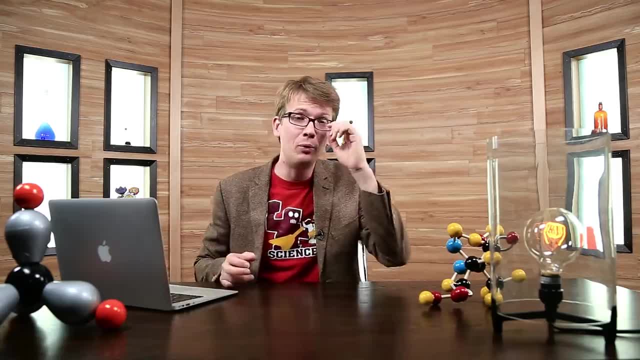 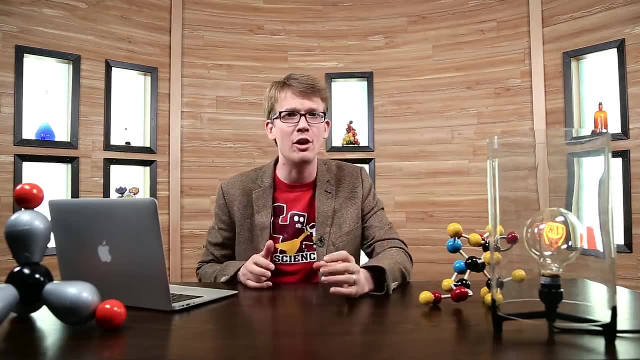 when the reactants rearrange into products. What the heck is this good for? Well, we can explain a mysterious thing, which is how reactions occur spontaneously in nature even though there's no energy given off, Or even they suck heat out of the environment and seem to go up the energy ladder instead. 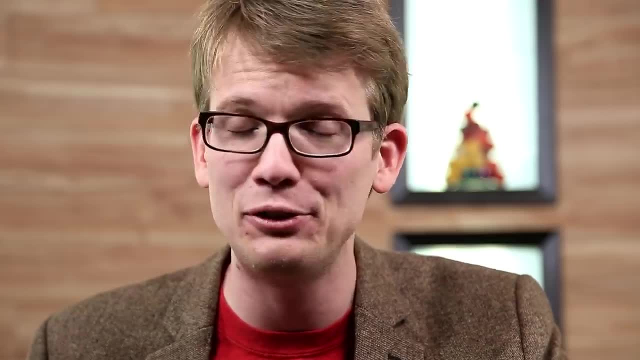 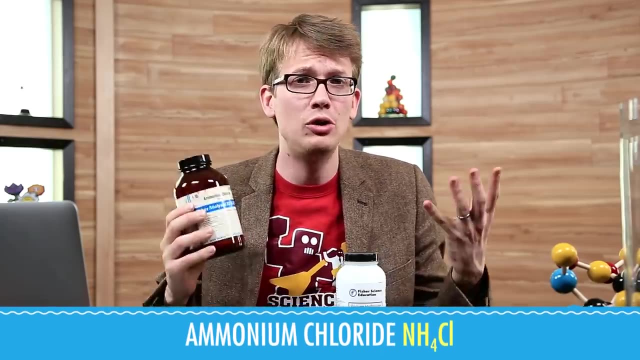 of down. Let's try it out with a real reaction here on my desk. This is one of my favorites. This is barium hydroxide octahydrate and this is ammonium chloride. Usually we do chemical reactions in aqueous solution because most solids don't interact. 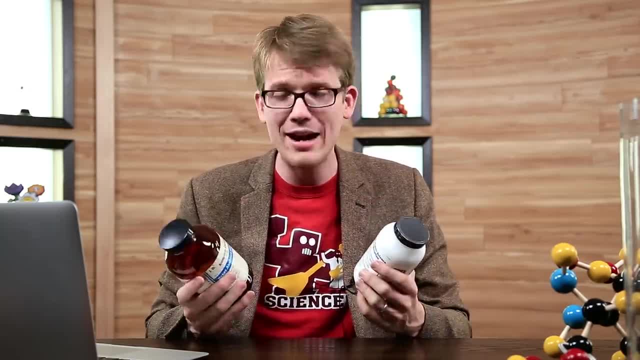 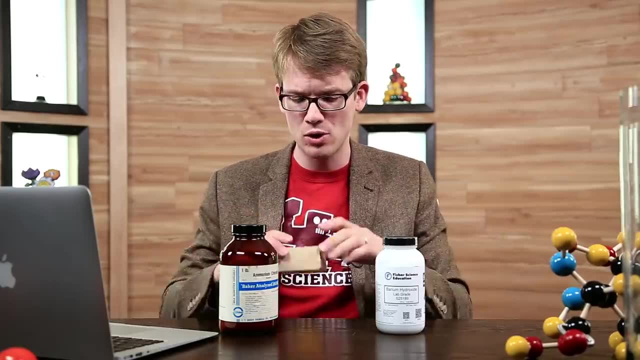 easily. but this pair is an exception to that rule. They react readily in solid form, And this reaction absorbs a lot of heat from the surroundings, making everything around it feel cold. Now, to show you how cold it gets, I'm going to do something here. 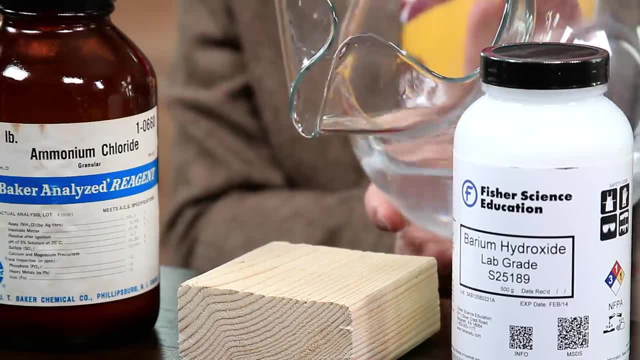 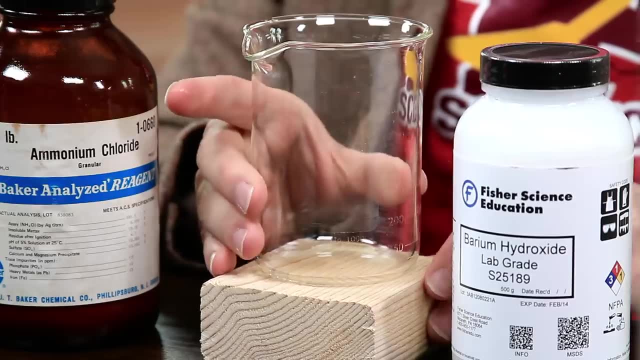 You're just going to have to assume you understand what I'm doing. What am I doing? What is happening? Why am I doing this? That's weird, Hank. Why are you doing that? And then I'm going to put that on there. 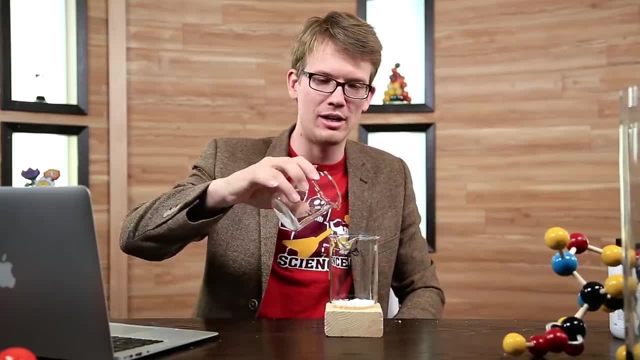 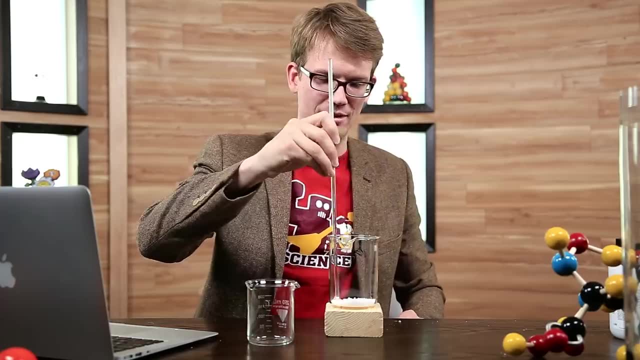 So I've got my barium hydroxide in this beaker. Now I'm going to dump the ammonium chloride in, And now one of the byproducts of this reaction is ammonia, so I'm going to have to smell that, but you don't. 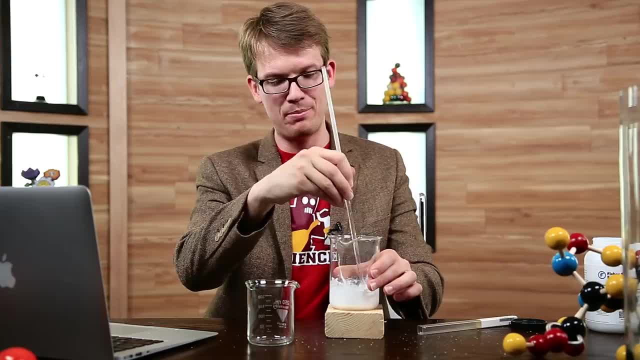 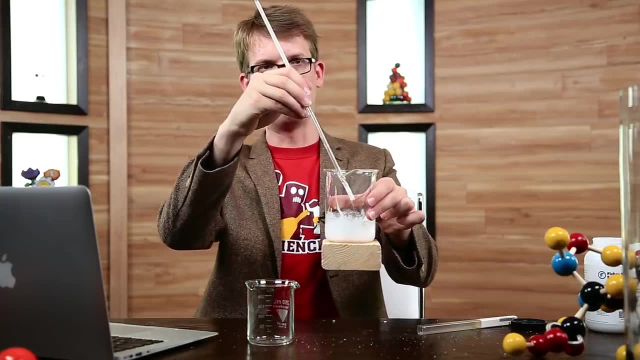 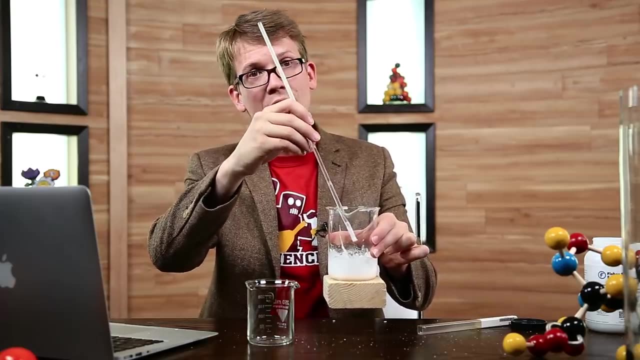 Oh yeah, Look at that slush. I think we've reacted pretty much completely here, And so we should, if all things have gone properly. yep, that's pretty cool. sucked enough heat out of the block of wood to actually freeze it to the beaker. 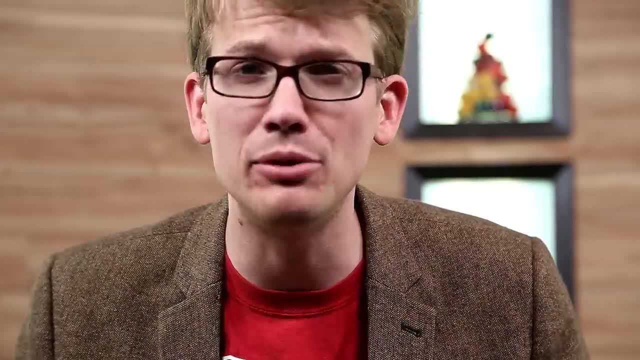 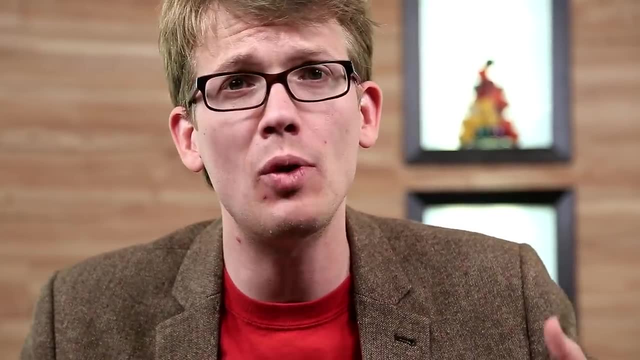 In the world of chemistry, a reaction that proceeds spontaneously and yet absorbs heat is really weird. Basically, I have a hard time believing what I just did. So what does entropy have to do with this little freak show? You might think it has something to do with taking the heat from the surroundings to make 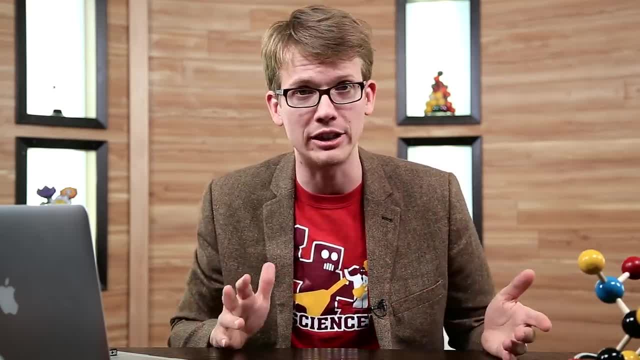 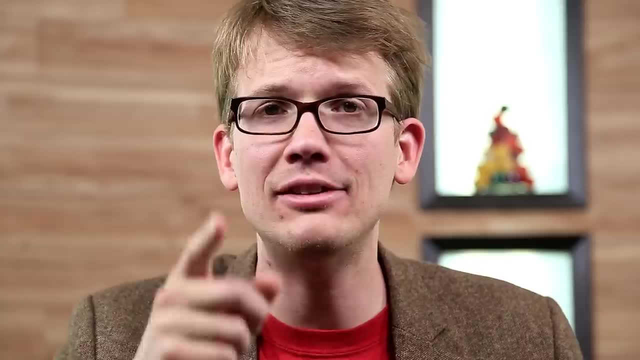 the system colder, but while that's counterintuitive and cool, that's not all of it. You might also think that it has to do with two solids combining to form a whole bunch more liquids and gases, and that is a big part, but still not all. 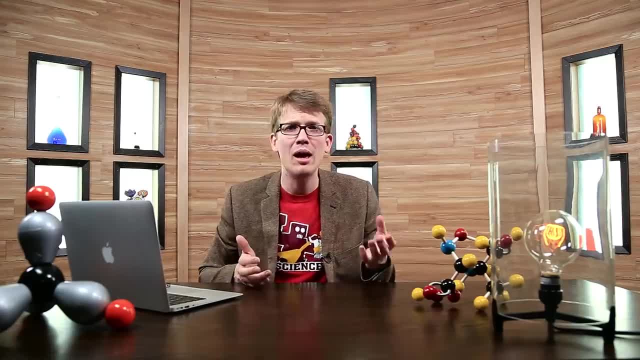 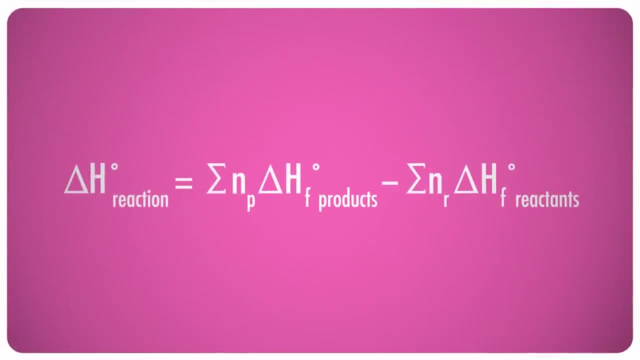 To understand what we just saw a little better, we need to put it all together. Let's start by finding out exactly how much heat it did absorb and what happened to the entropy as well. First, we'll find the enthalpy change, using Hess's law, in standard enthalpies of formation. 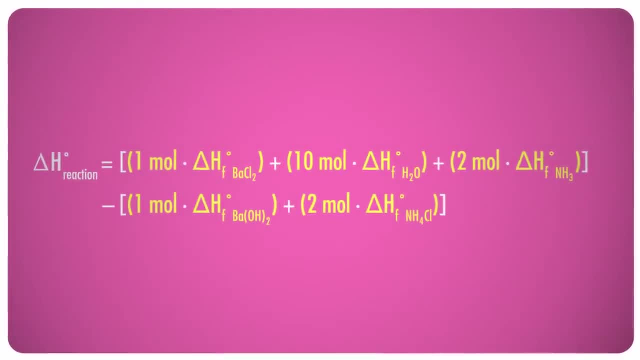 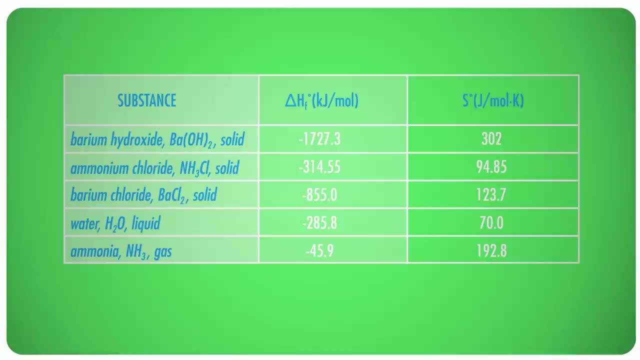 We can use the coefficients from the balanced chemical equation to fill in the number of moles for each substance. Then we have to look up a whole bunch of numbers, Remember. you can find tables like this online and probably in the back of your chemistry. 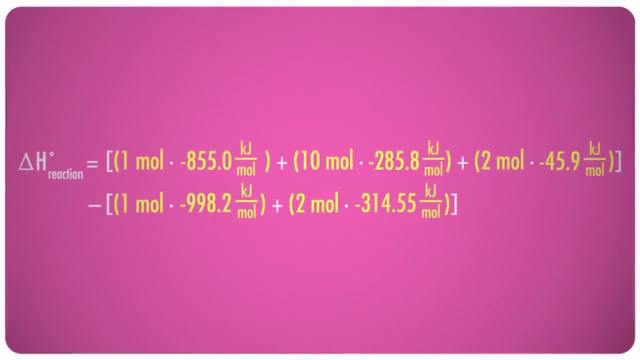 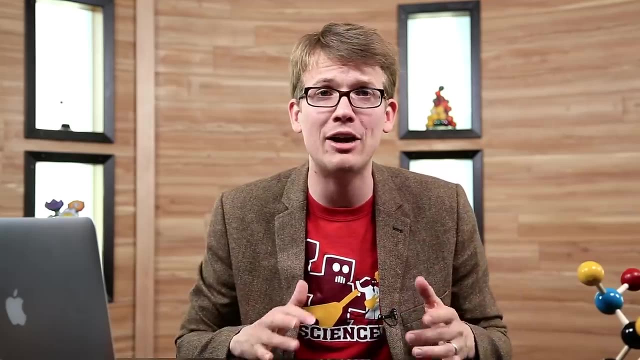 textbook too. When we plug the standard enthalpies of formation into the formula and do the math, we find that the change in standard enthalpy is plus 166 kilojoules. It's positive, which makes sense because the reaction absorbed the thermal energy enough. 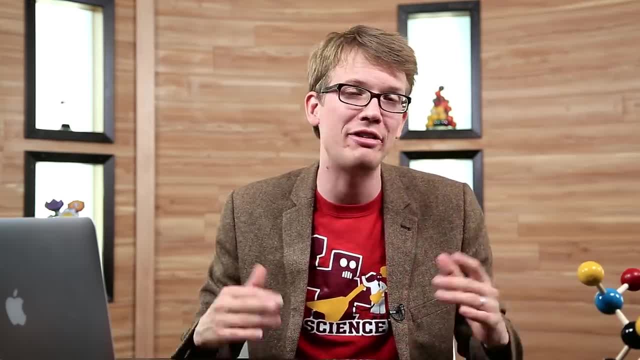 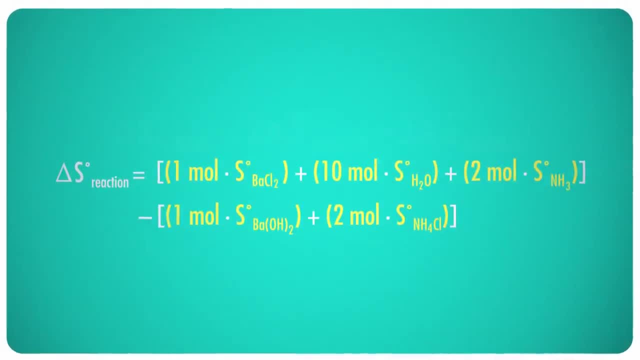 to create about a half a kilogram of ice if it had been surrounded by water instead of air and fingers. Next we'll find the entropy change. Remember the basic equation is the same. We put in the number of moles from the balanced chemical equation and the standard entropies. 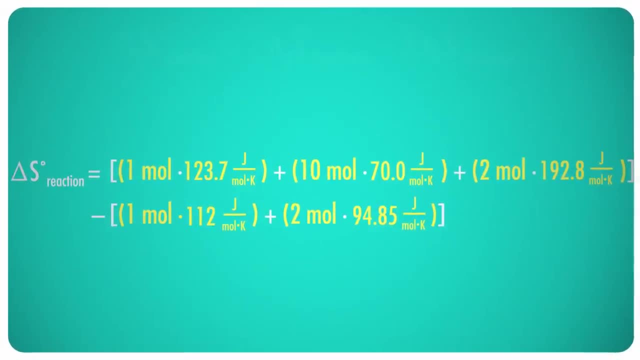 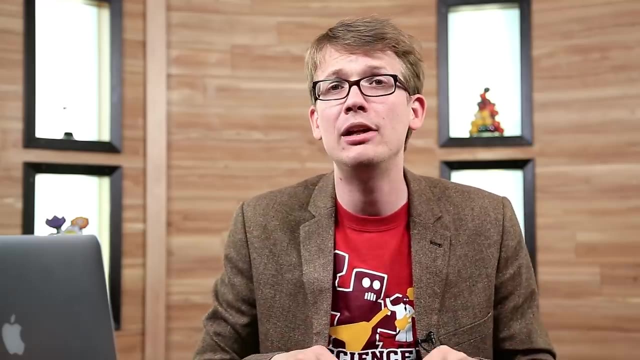 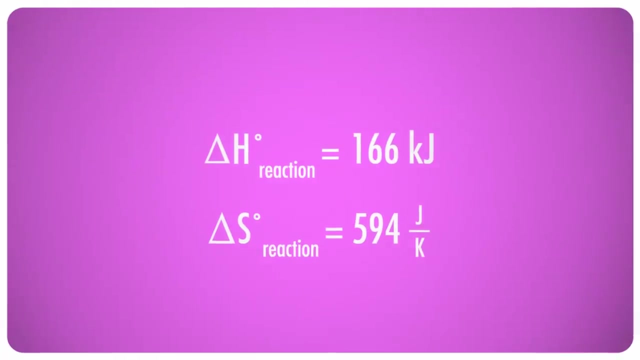 from a table and a quick calculation tells us that the change in standard entropy is 594 joules per kelvin. A positive result means the entropy of the reaction increased, meaning the products were more disordered than the reactants. Note that the standard enthalpy is in kilojoules, while the standard entropy is in joules per. 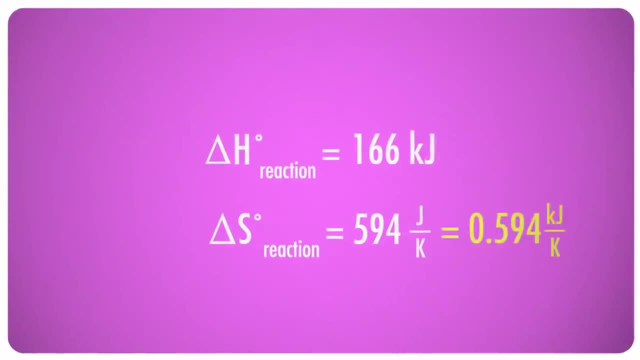 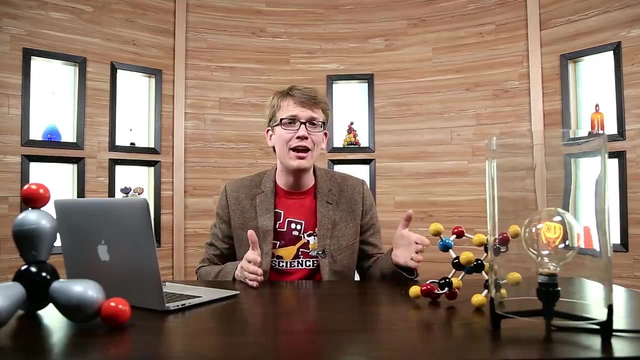 kelvin, The energy units should match, so let's call the standard entropy 0.594 kilojoules per kelvin. That doesn't look like much right now, but wait, there's more. Those numbers don't explain why the reaction proceeds spontaneously, even though it scavenges. 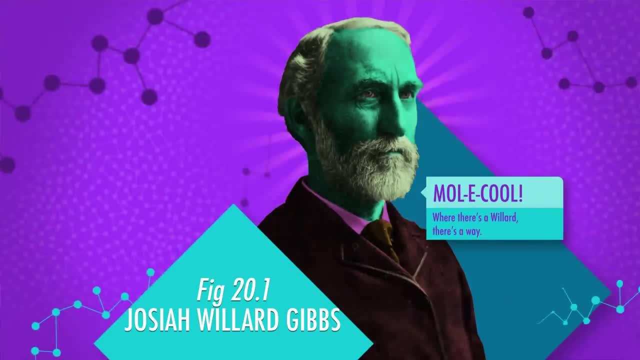 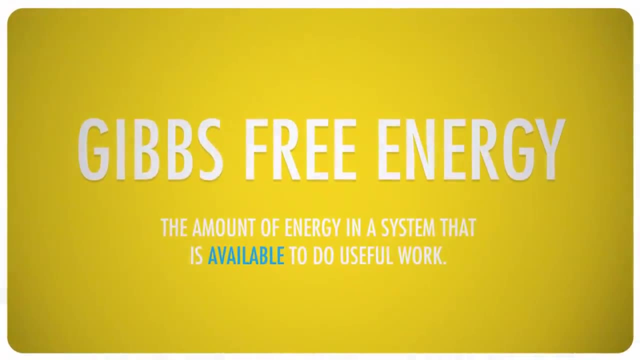 all that heat from the environment. But Josiah Willard Gibbs- he found a way to explain it and he didn't even mean to- Gibbs was interested in the amount of energy in a system that was available or free to do useful work. 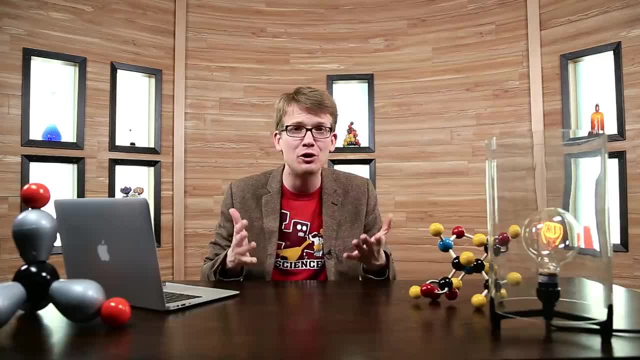 Today we call this Gibbs free energy, or sometimes the standard free energy, or simply free energy of the system. Like enthalpy and entropy. Gibbs free energy is a state function. It's a state function of energy. It's a state function of energy. 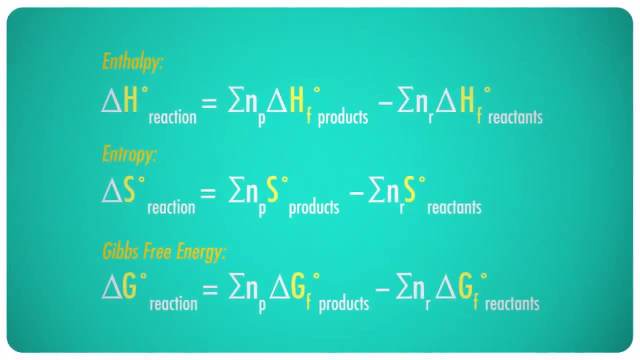 It's a state function, so it can be calculated the same way. We simply substitute delta G, which stands for Gibbs free energy, for delta H or S. The standard free energy of formation, written like this, is the change of free energy that. 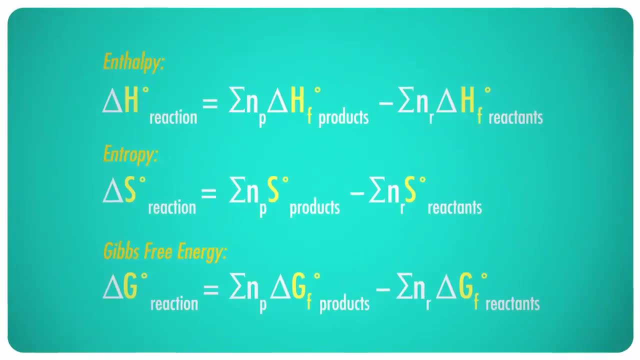 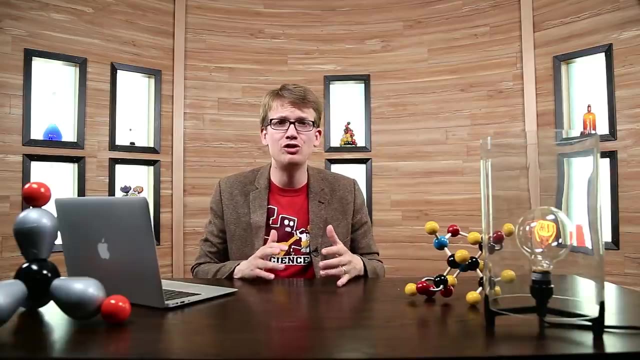 occurs when a substance is formed from its elements in a standard state. It's analogous to the standard enthalpy of formation that we use to calculate change in enthalpy. Like enthalpy and entropy, we can't directly measure the free energy change of a whole. 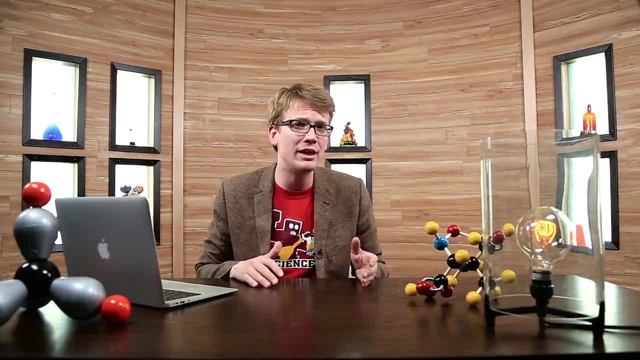 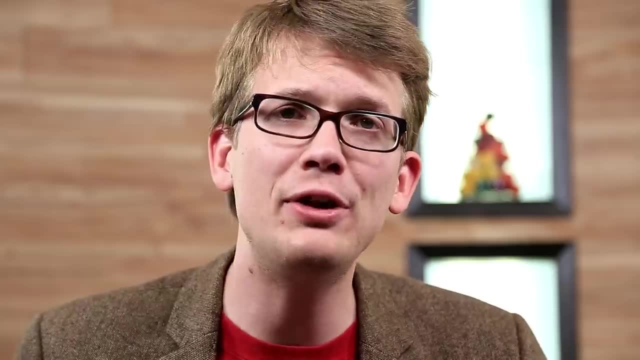 reaction. So scientists created a baseline by setting the standard free energy change of formation for an element In its most stable form, at standard state, to zero. The standard free energy change of formation for a compound, then, is just the difference between its standard free energy and that baseline. 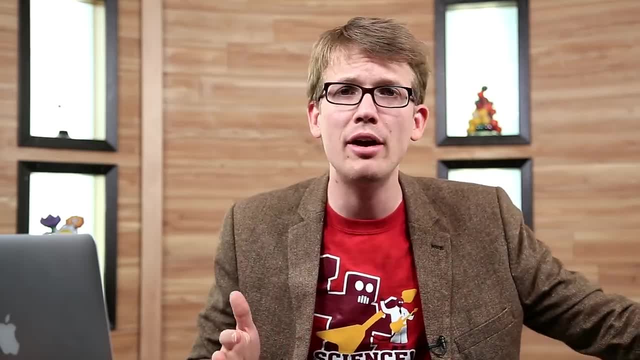 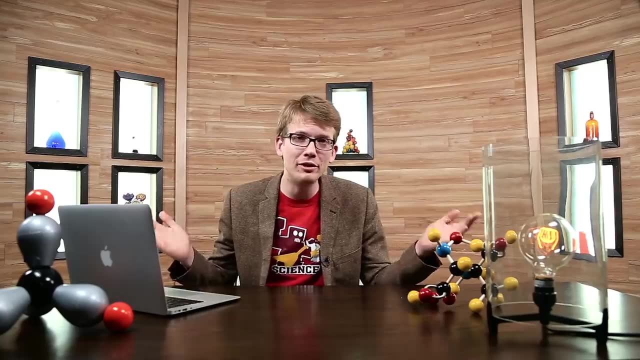 But what if you don't know the standard free energies of formation for the products and reactants? Well, they're often listed in tables, but sometimes the ones you need aren't available. Never fear, Willard Gibbs has an app for that. 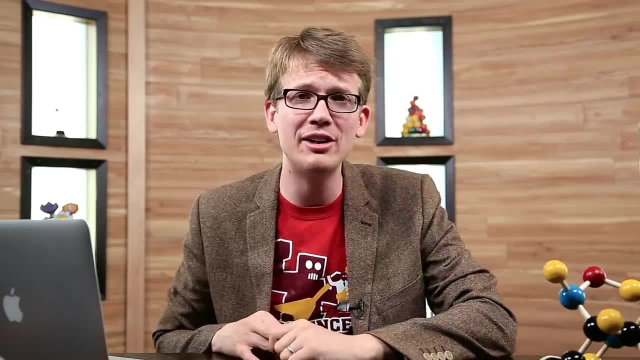 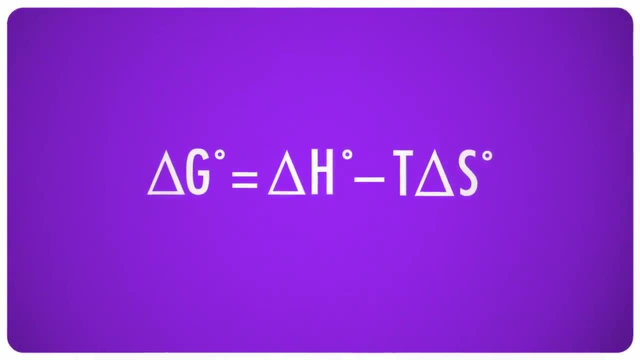 It's actually a formula, But he figured it out In 1873,. Gibbs calculated that at constant pressure and temperature, the change in the standard Gibbs free energy for a reaction equals the change in standard enthalpy minus the product of the temperature and the change in standard entropy. 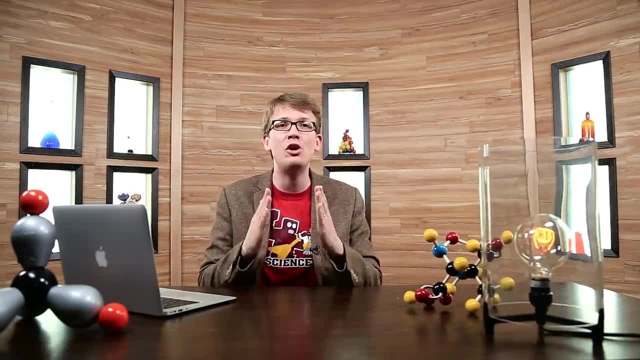 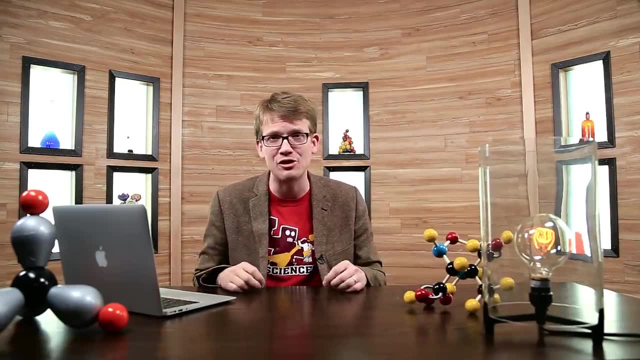 In other words, the amount of free energy a reaction makes available to do work depends on two and only two things: The enthalpy change, the amount of heat the reaction transfers, and the entropy change, the amount of disorder it creates at a given temperature. 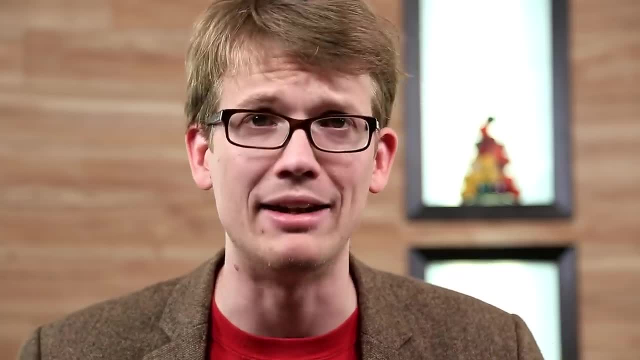 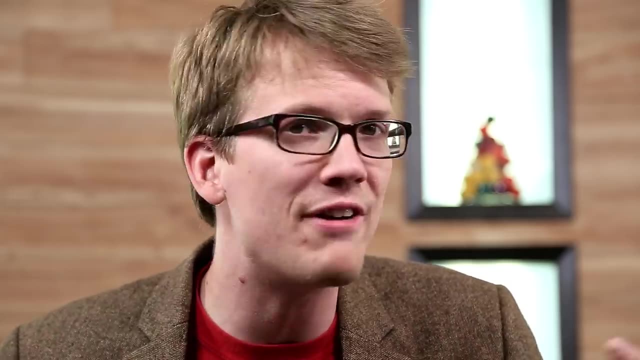 So which is more important, The heat transfer or the disorder? Well, it depends. A large change in enthalpy can determine the direction of a free energy change, And that's what we're looking for. If the absolute value of the change in enthalpy is greater than the absolute value of the 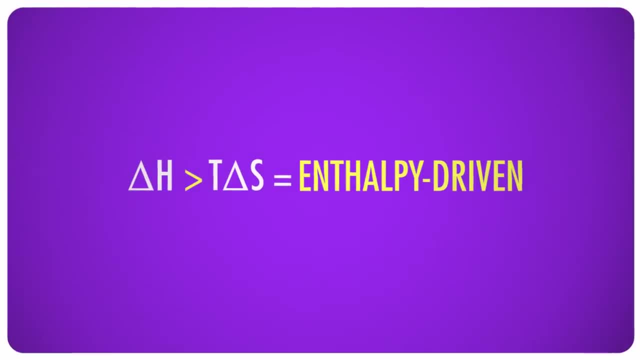 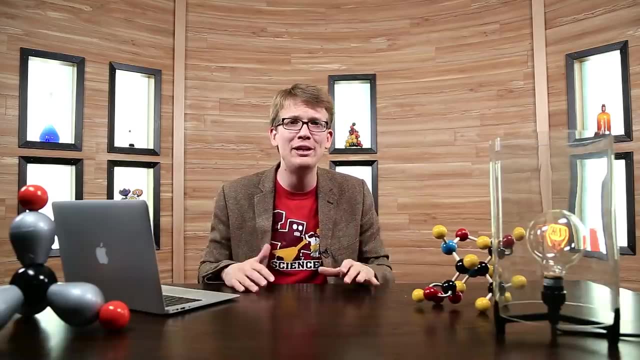 product of the temperature and the change in entropy, or T-delta-S, then we say that the reaction is enthalpy-driven. This means that the flow of thermal energy provides most of the free energy in the reaction. On the other hand, if the absolute value of T-delta-S is greater than the absolute value, 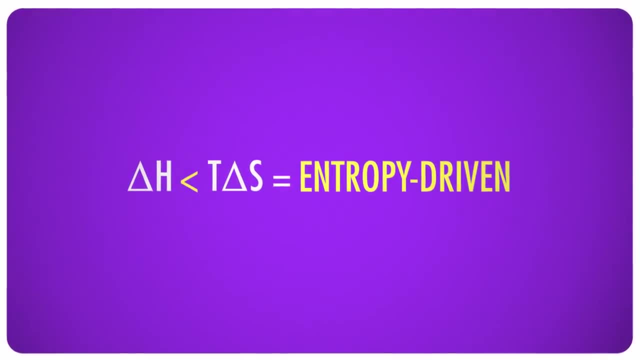 of the enthalpy change. we call the reaction entropy-driven, meaning increased disorder provides most of the reaction's free energy. Which type was the barium-hydroxide reaction? Well, I'm gonna say that the temperature in here is about 25 degrees Celsius, or 298.15. 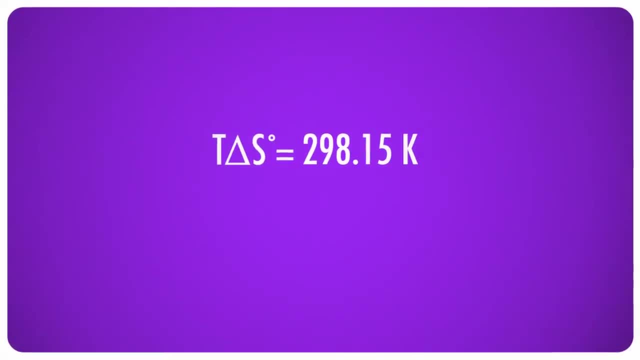 Kelvin, because I'm awesome like that, I can just tell: When we multiply that by the change in entropy- that we calculated 0.594 kilojoules per Kelvin- we get a value of 177 kilojoules. If we compare that to the change in enthalpy, we calculated 166 kilojoules. it is clear. 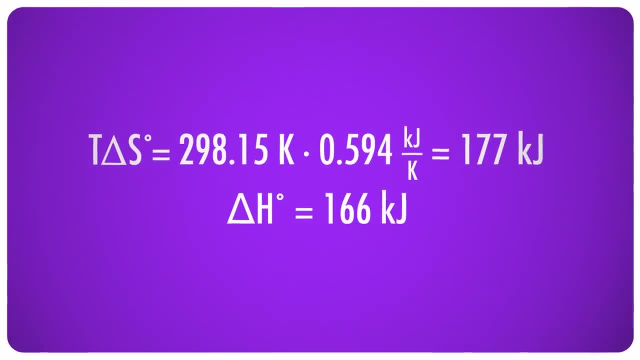 that the T-delta-S is higher than the delta-H. So the reaction is entropy-driven. So we get a value of 177 kilojoules per Kelvin. If we compare that to the change in enthalpy, we calculated 166 kilojoules. it is clear that the T-delta-S is higher than the delta-H. 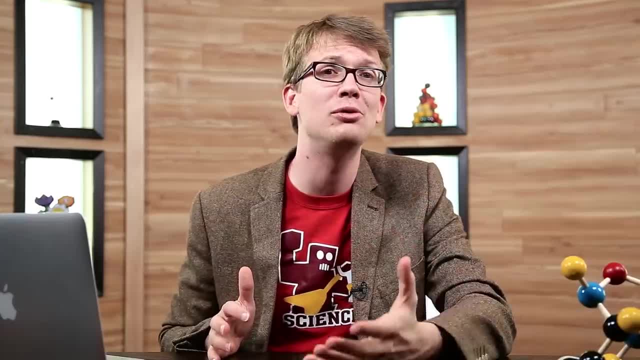 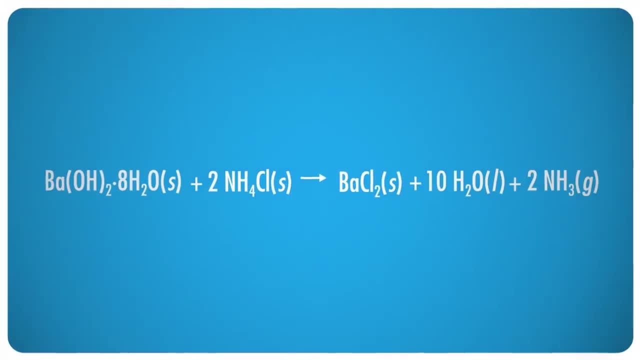 So the reaction is entropy-driven. no surprise there: Even though the reaction absorbed a lot of thermal energy, this phenomenon was dwarfed by the increase in entropy. And this makes sense, because the balanced equation goes from three total moles of solids. 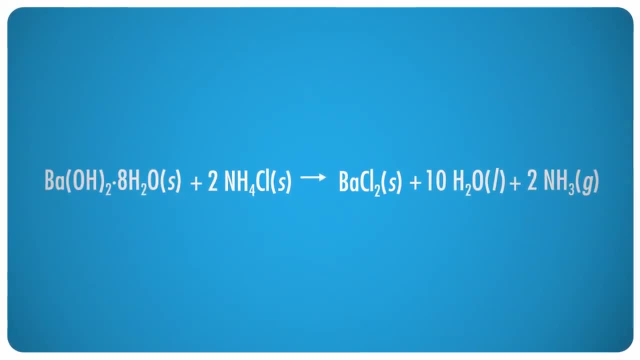 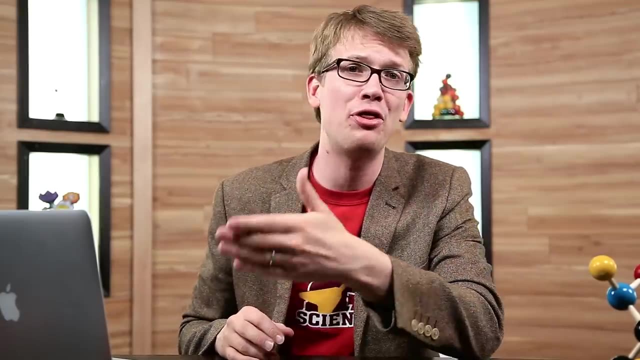 with their molecules locked in place to one mole of solid, ten moles of liquid and two moles of gas. This is a massive increase in disorder because, in addition to the fact that there are now thirteen moles of particles to move around instead of just three- the liquid and gas- 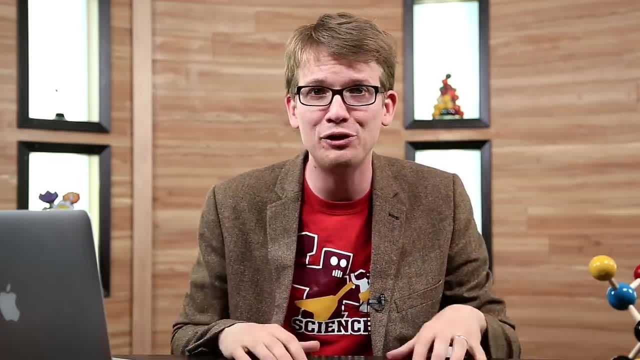 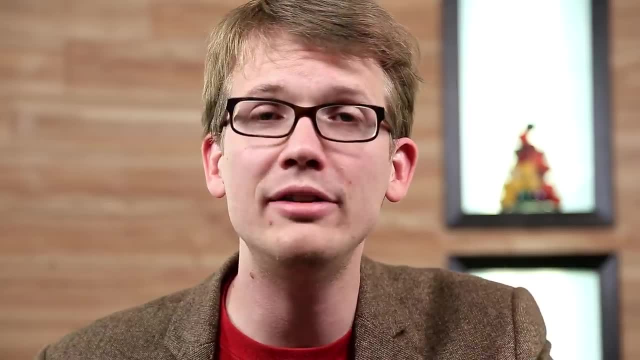 are particularly good at moving around, So most of those particles are in random motion, no longer stuck in one spot, causing a large increase in disorder or entropy. But here's the coolest part: Gibbs' formula also tells us whether the reaction is spontaneous. 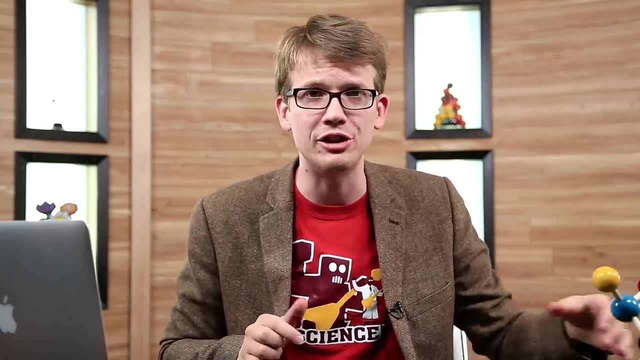 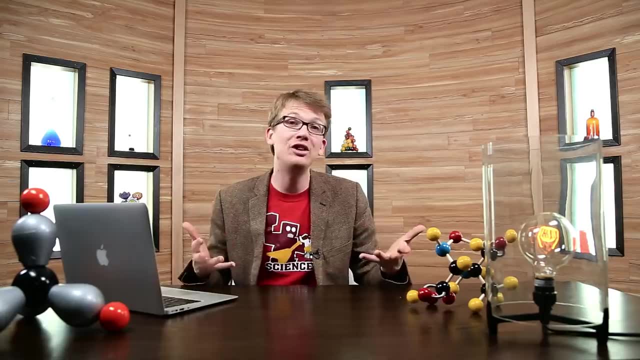 or not, We know all systems tend toward the lowest possible energy state, whether it's a ball rolling down a hill, elastics springing back into shape, or positive and negative ions forming a bond. Delta-G is a type of energy, obviously, so it spontaneously approaches the minimum possible.